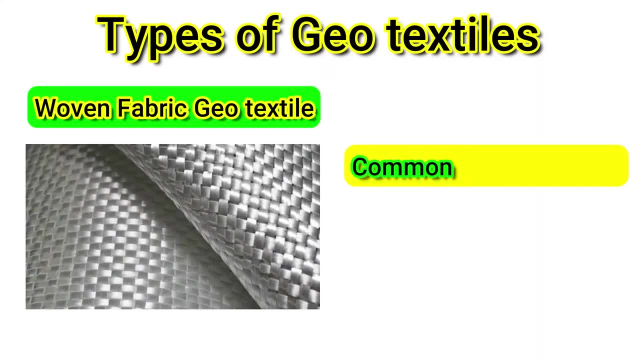 They are the common geotextile type and they are manufactured by weaving like usual clothing. They consist of two parallel threads or yarns. The next type is nonwoven geotextile. This is what is shown in this particular photograph. 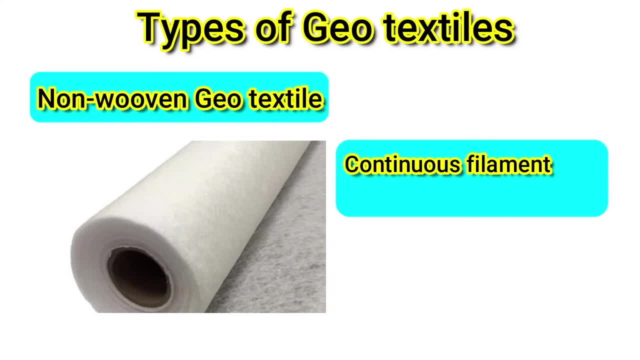 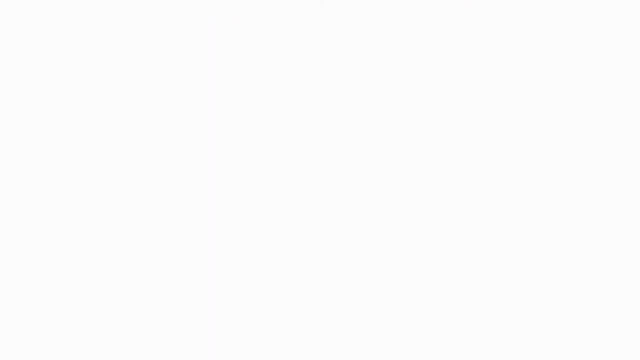 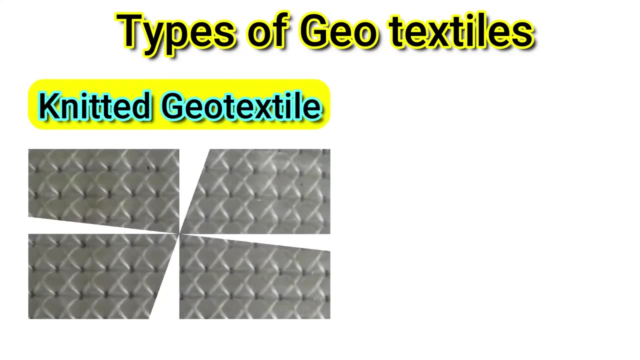 They are continuous filament yarn or short staple fiber. They are bonded using thermal, mechanical and chemical methods. The next type of geotextile is knitted geotextiles. They are manufactured by interlocking a series of loops of yarn together. 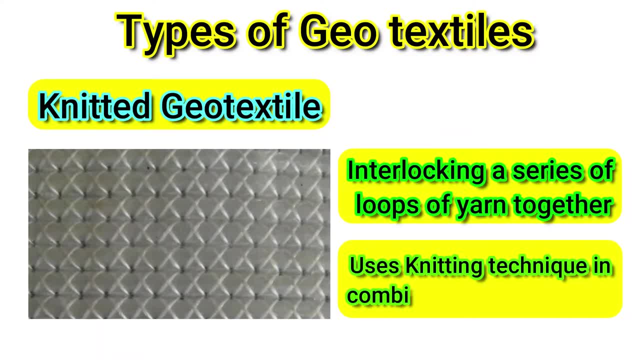 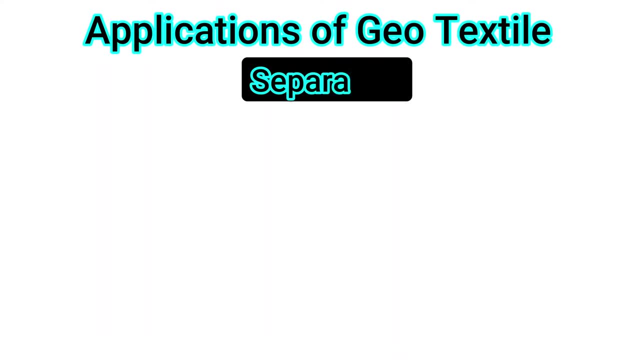 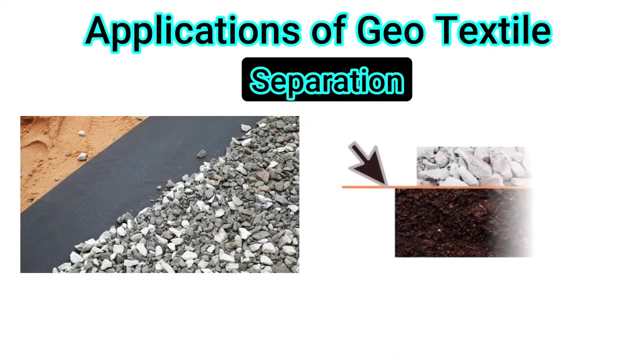 They uses knitting technique in combination with weaving. What are the applications of geotextiles? The first one is separation. They act as a separator. This is the typical cross section of a road. This is the base course, and below that comes the subgrade soil. 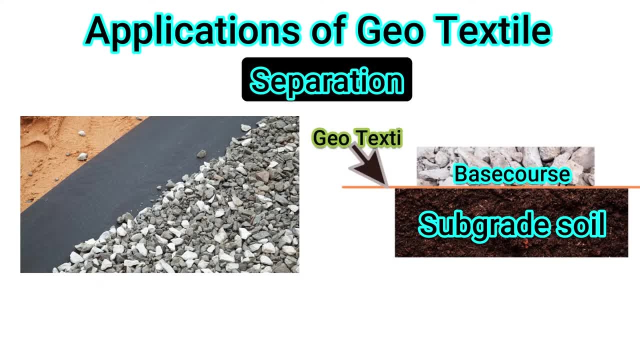 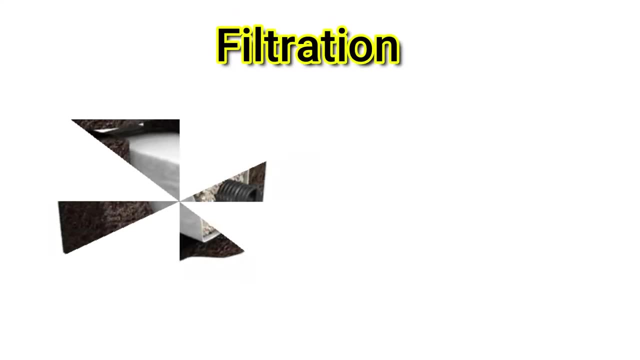 Geotextile is placed between the base course and the subgrade soil and they prevents intermixing of fine subgrade soil with aggregates of base course or GSP. Next major application is filtration. They are used in filtration. They are used in filtration of walks and they allows adequate liquid flow with minimal loss. 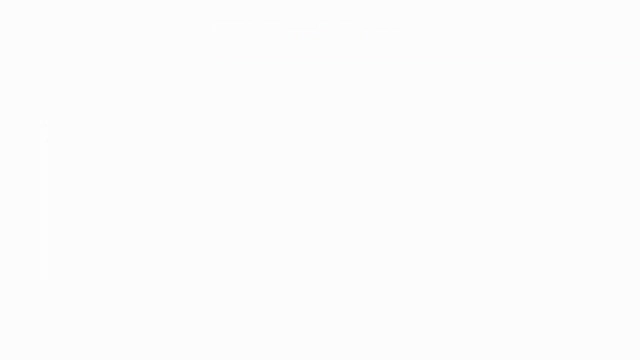 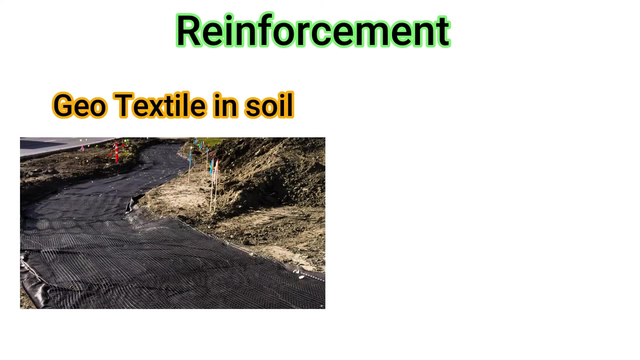 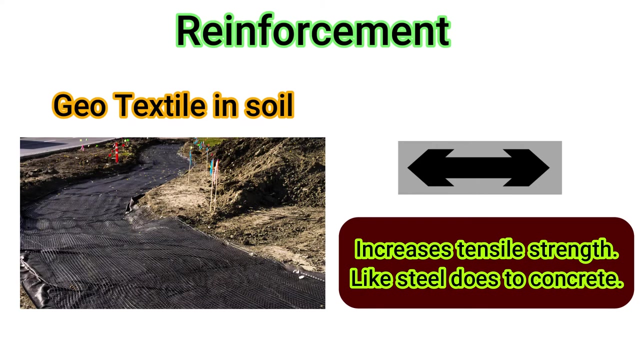 of soil. What are the applications of geotextiles? They acts as reinforcement. Geotextile acts as reinforcement. that is mainly for road structures, and geotextile in combination with soil acts as a reinforcement. They increases the tensile strength, just like steel does to concrete. 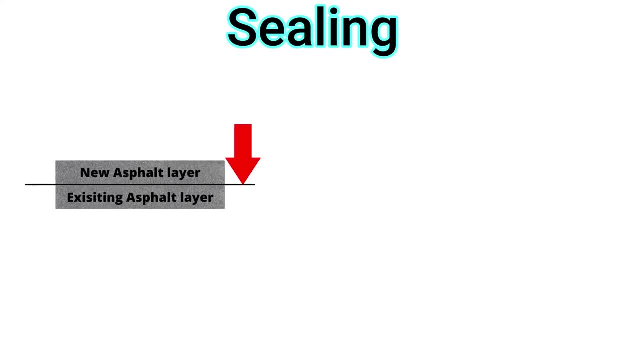 What are the applications of geotextiles? Geotextiles are used for sealing applications. This is the typical old and new asphaltic layer cross section. They are provided between old asphalt and new asphalt surface. Geotextile is used for drainage purpose. 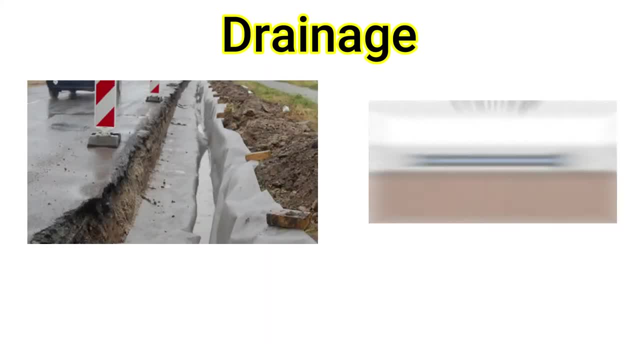 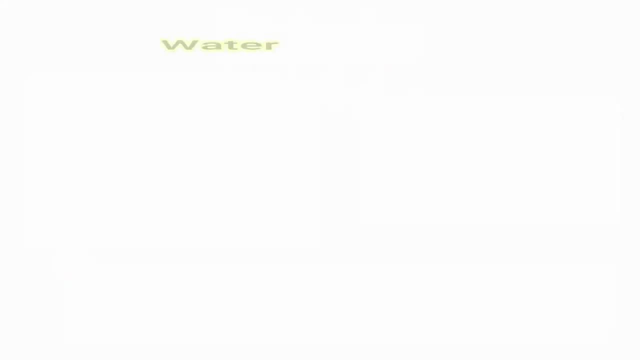 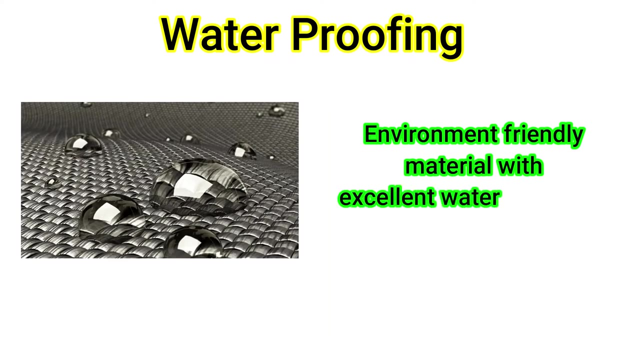 They are used for road side drains. The main purpose of geotextile is they are used to remove moisture or fine particles from the system. Next major application is in the waterproofing sector. They are extensively used in waterproofing. They are environmental friendly material with excellent waterproof and anti seepage performance. 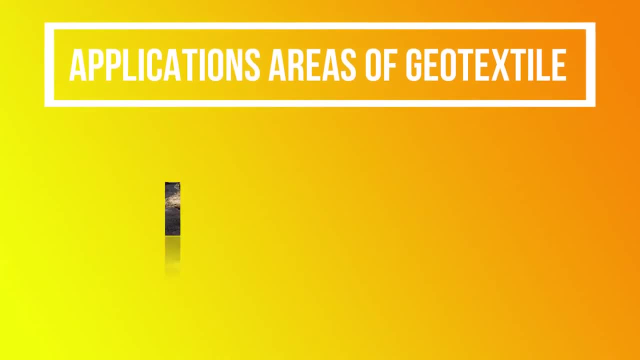 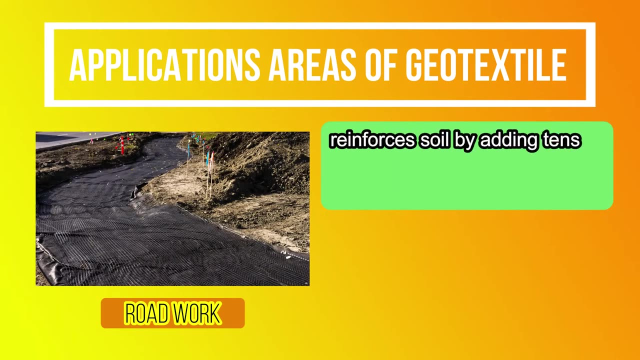 Areas of applications of geotextiles. where geotextiles are used? A major usage is in road works. They reinforces soil by adding tensile strength, Acts as a rapid dewatering layer, Acts as a permeable layer and separated between the road layers. 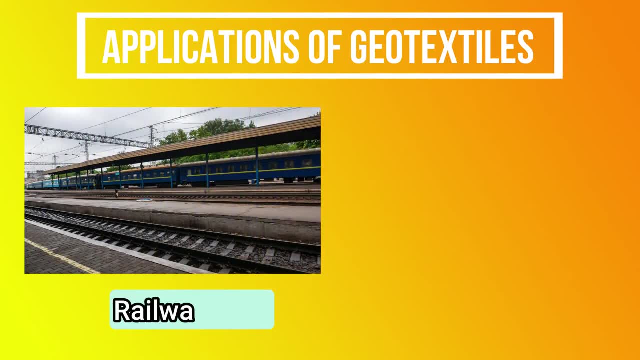 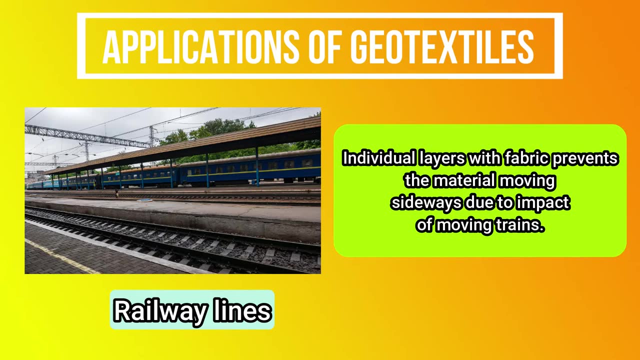 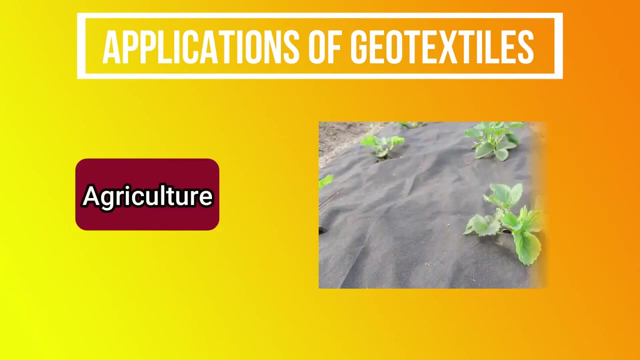 They are used for railway lines. The individual layer, separated with the fabric, prevents the material moving sideways due to the movement of trains. They are used in drainage works. They are used in the agriculture sector. They are used for canal and river slope protection works. 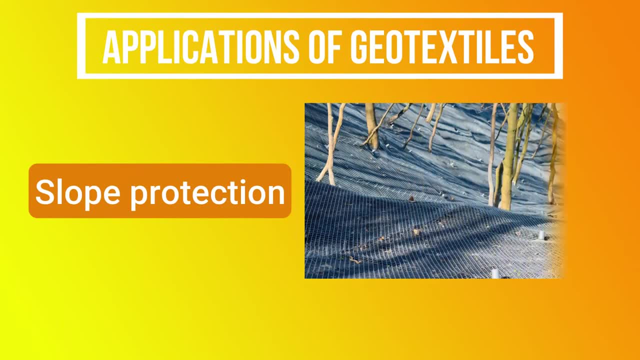 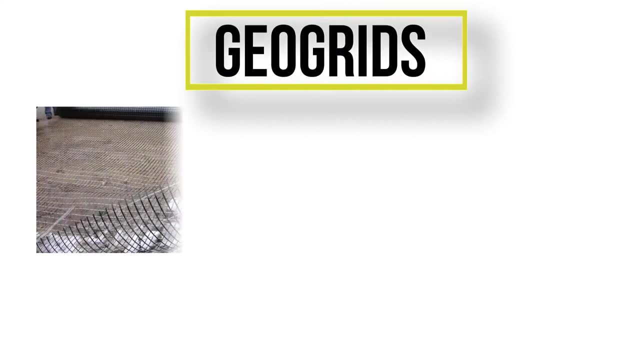 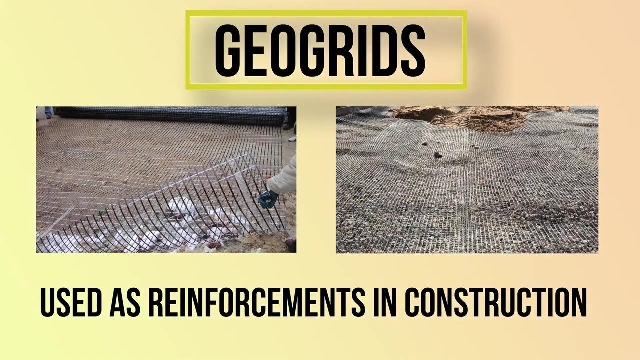 They are also used for slope protection and stabilization of soil. Next major use is in the drainage works. They are used in the drainage works. Next major geosynthetic type is geogrids. Geogrids are mainly used as reinforcements in construction. 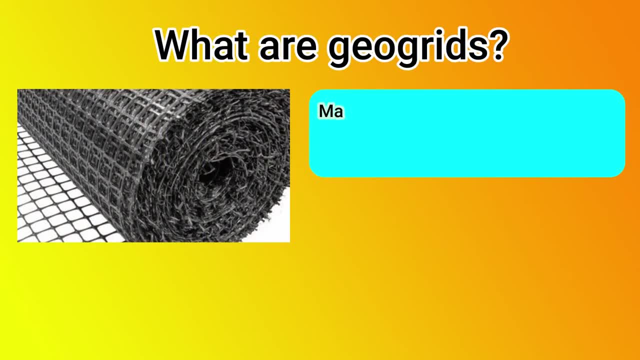 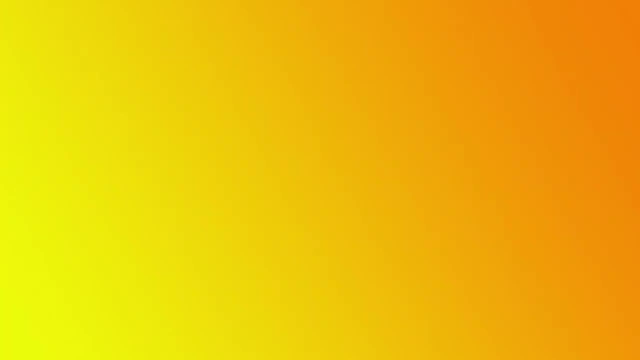 What are geogrids? They are manufactured from polymer materials like polypropylene, polyethylene or polystyrene. They are manufactured from the extrusion, weaving or welding process. They are in the form of open grids, as shown in this photograph. 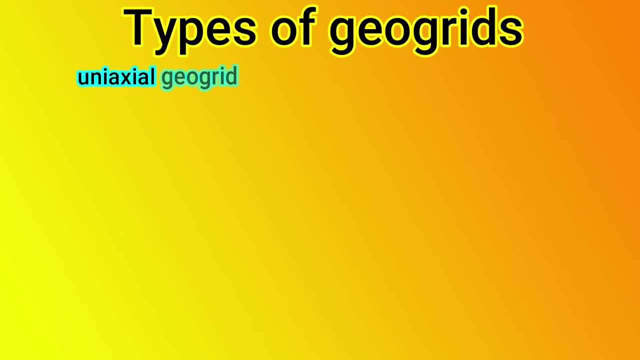 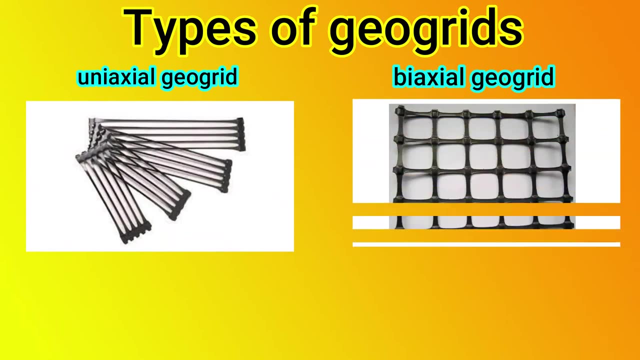 What are the types of geogrids? First one is uniaxial geogrids and the second one is biaxial geogrids. Uniaxial geogrids are formed by stretching of ribs in the longitudinal direction. 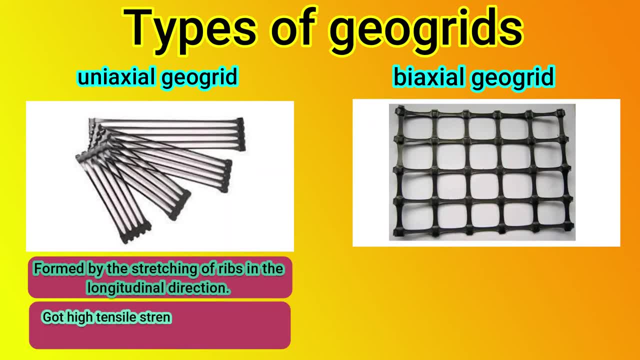 They could hide tensile strength in the longitudinal direction than on the transverse direction. Biaxial grids are formed by punching of polymer sheets. The stretching is done in both directions. The tensile strength is equally given to both sides. The tensile strength is equally given to both sides. 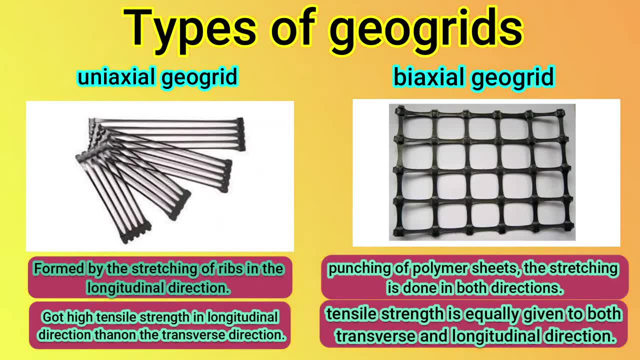 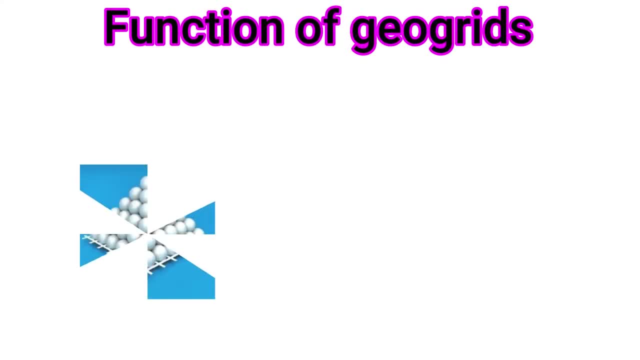 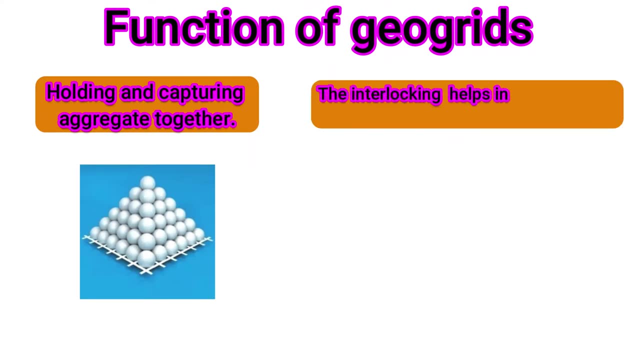 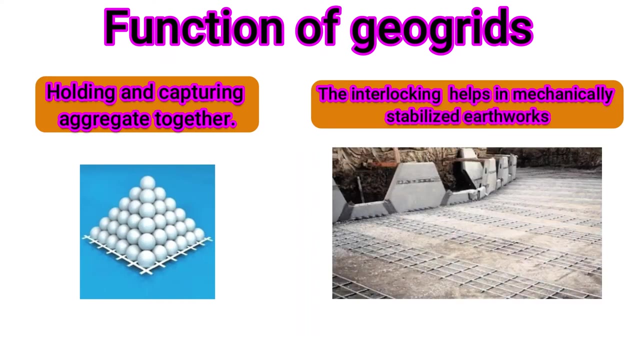 The tensile strength is equally given to both sides. What are the functions of geogrids? They are capable of holding and capturing the aggregates together. The interlocking helps in mechanically stabilized earthwork. The next French was the function of geo-grides. 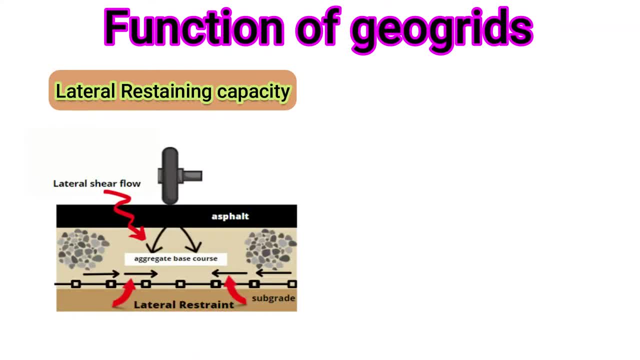 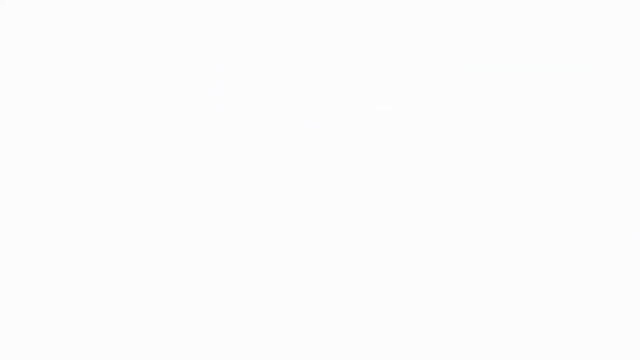 They can act lateral or they got good lateral restra así capacity. this is a wheel load coming down and it tends to slide the aggregates to the sides, but the geogrids can act as lateral restraint and they improve the bearing capacity and reduces the lateral movements of the aggregate, just as shown in this figure. 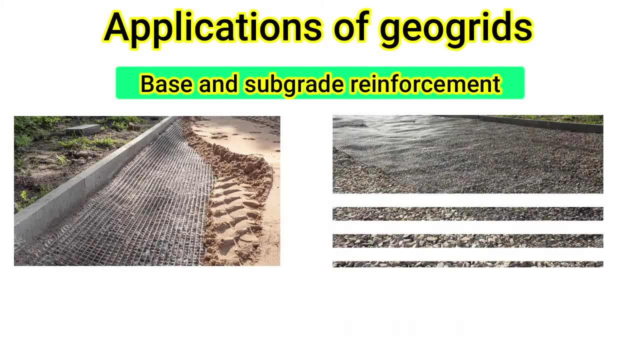 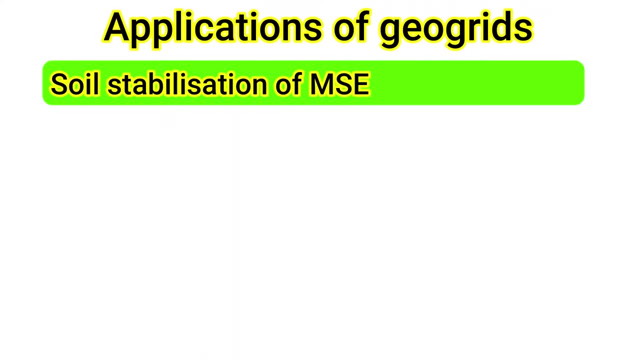 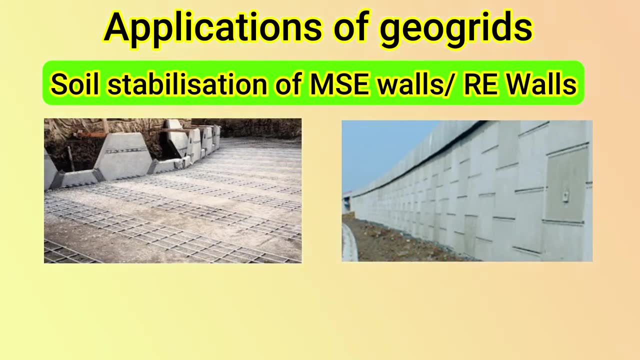 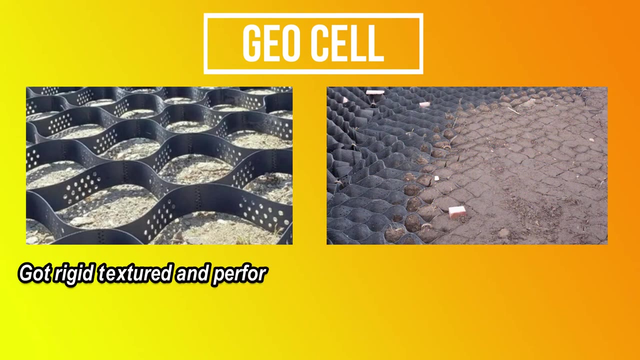 next is they are used for base and subgrade reinforcement in roads. they are used for soil stabilization of msc walls or re walls, that is, mechanically stabilized earth walls. the next major type of geotextile is geocell. they got rigid, textured and perforated walls of a flexible 3d cellular mattress. they are extruded. 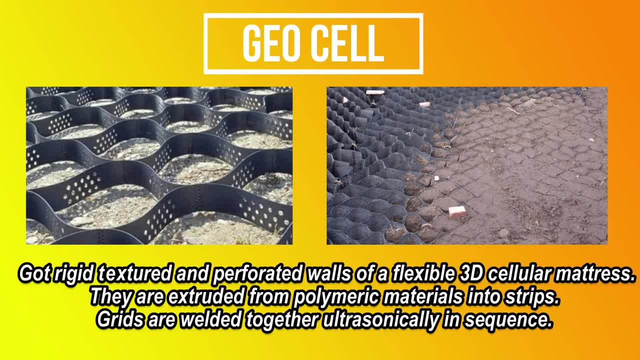 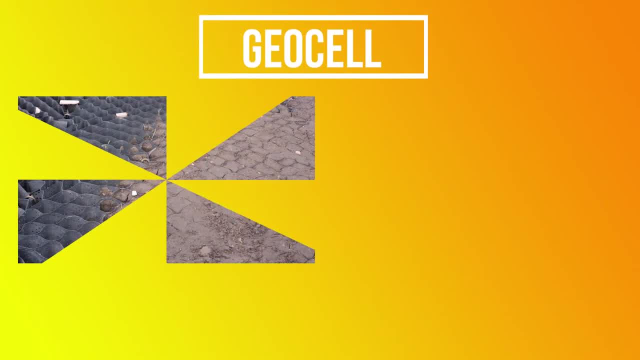 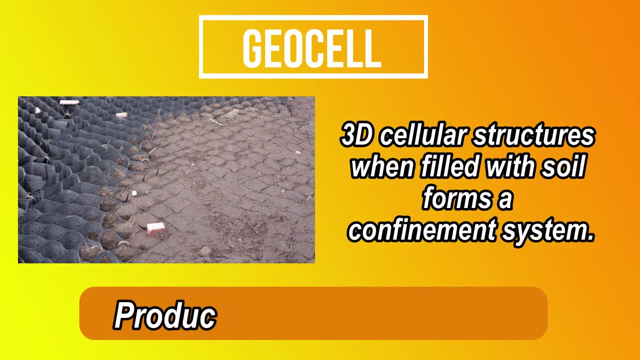 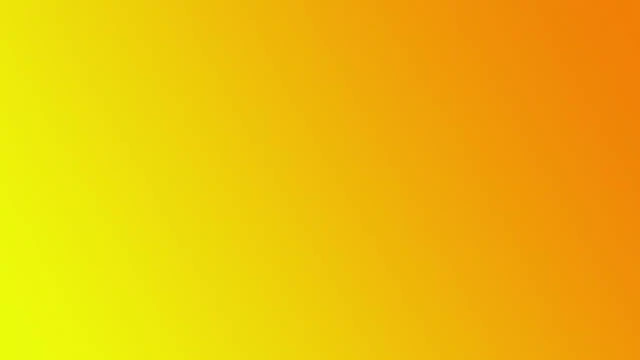 from polymeric material into strips and are joined together ultrasonically in sequence. their function include this: 3d cellular structures, when filled with soil, forms a confinement system. they produces a composite layer. next is geonet. they consist of ribs at two horizontal planes. that is separate, separate. 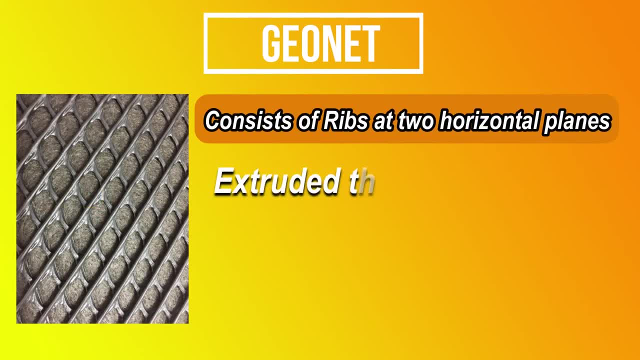 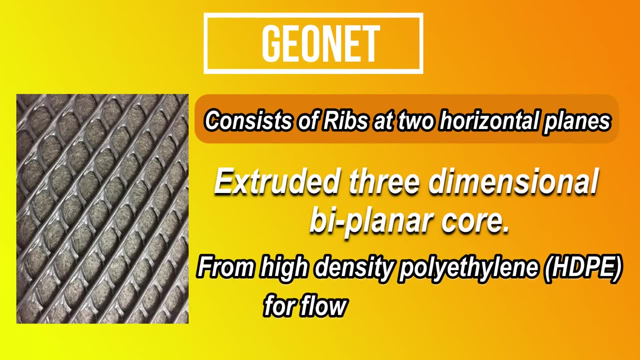 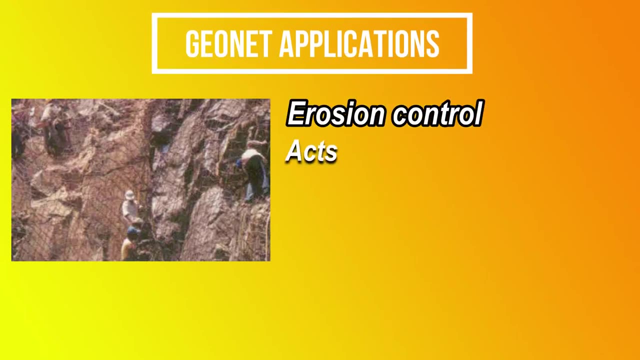 planes. they are extruded three-dimensional bi-planar core they they are manufactured from high-density polyethylene, that is for flow under high density. geonet applications include erosion control. they acts as check dams, control surface runoff, use in drainage layers for making water flow in the grid. 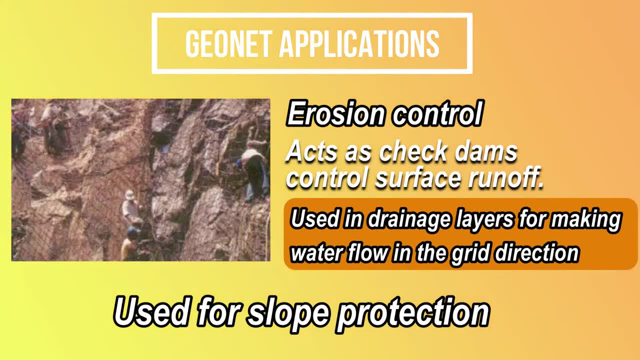 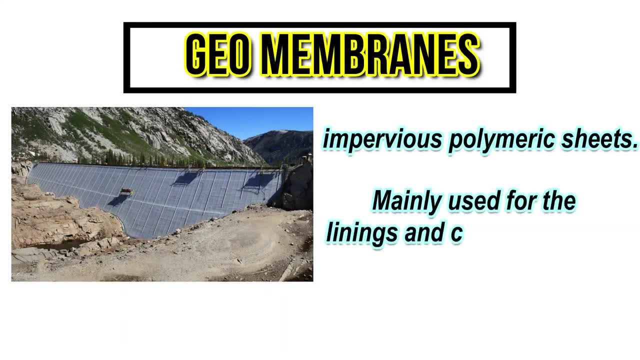 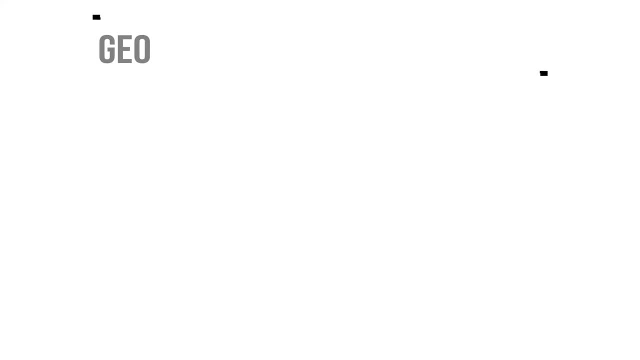 direction, use for slow protection, etc. next is geomembranes. they are impervious polymer sheets mainly used for the lining and covers of liquid and storage facilities. next is the application of geomembranes. they are used in landfill and canal lining. they are also used for 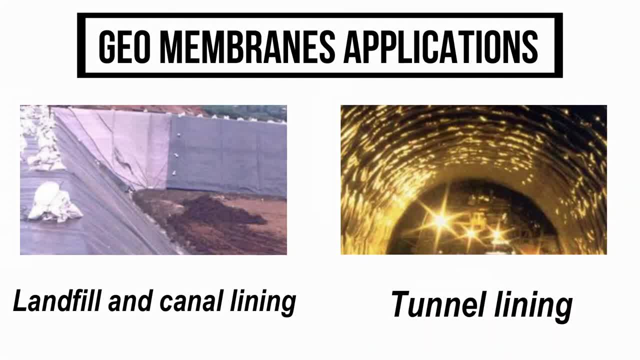 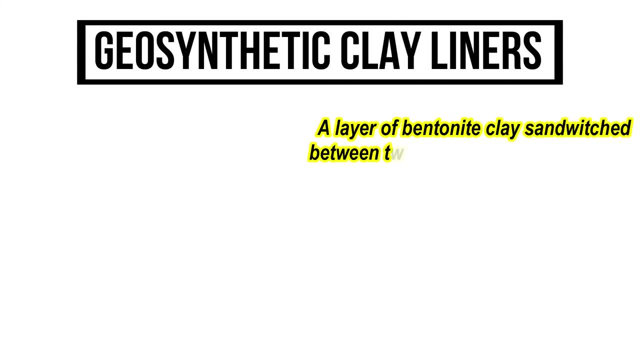 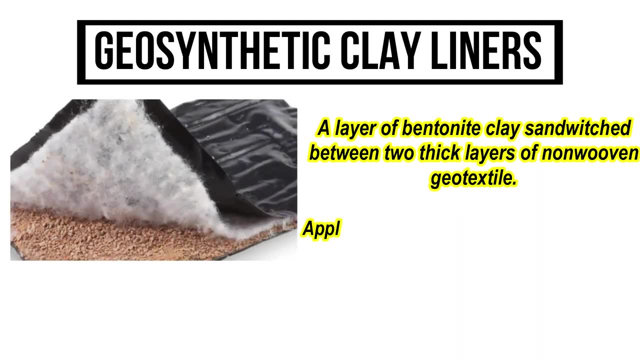 tunnel lining. next is geosynthetic clay liners. they consist of a layer of bandonite clay sandwiched between two layers of non-woven geotextile. they are applied below and above geomembranes. the main application include self-repair bandonite.